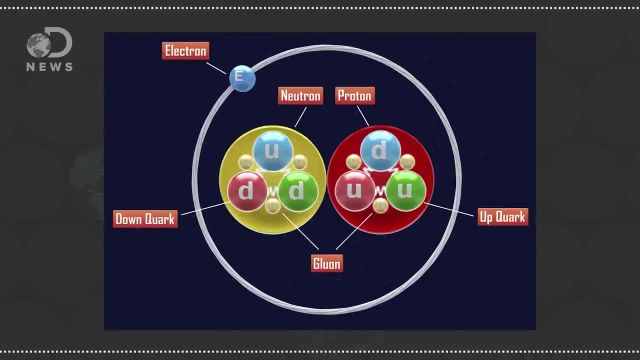 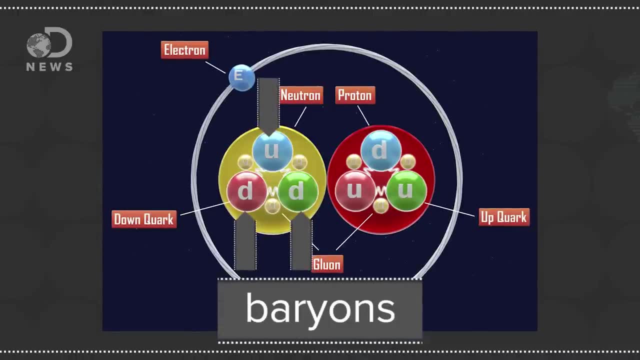 But they also come in colors. To build a particle it has to be color neutral, So you either need three quarks that are red, green and blue. Those particles are called baryons, and a proton is one of them. 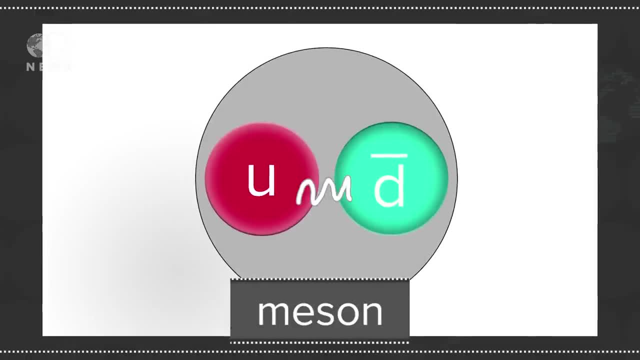 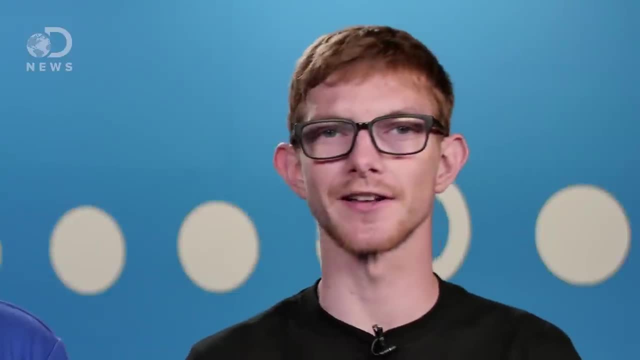 Or a meson is made when a quark and anti-quark- that are opposite colors- combine Like red. and what's the opposite of red Anti-red? You're so literal, I love it And you're also completely correct. Separate from quarks. you have leptons. 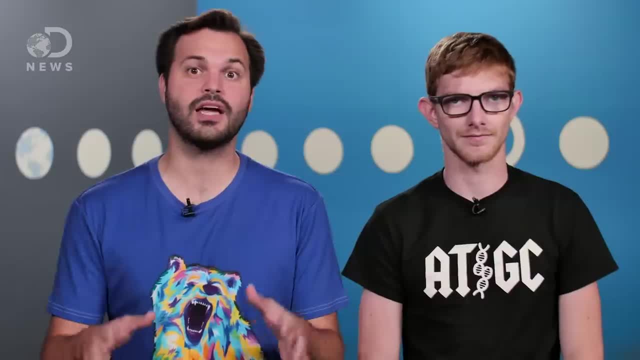 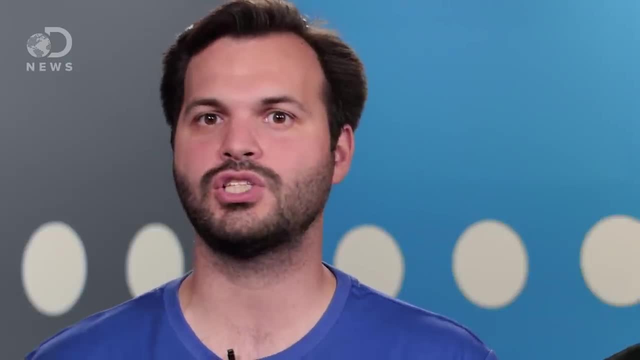 Like electrons and neutrinos, These are very, very light. An electron weighs in at just half an electron volt, So their name actually comes from the Greek word for light. Now quarks can change into other quarks, and leptons can change into other leptons. 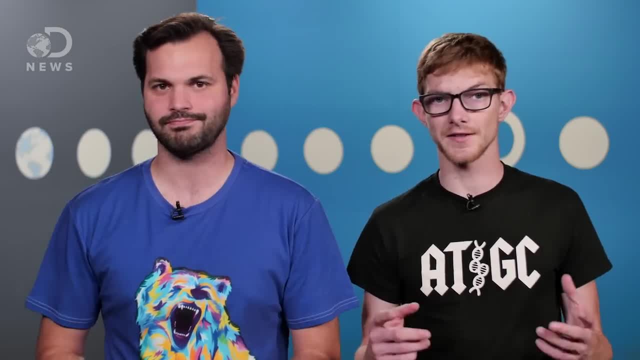 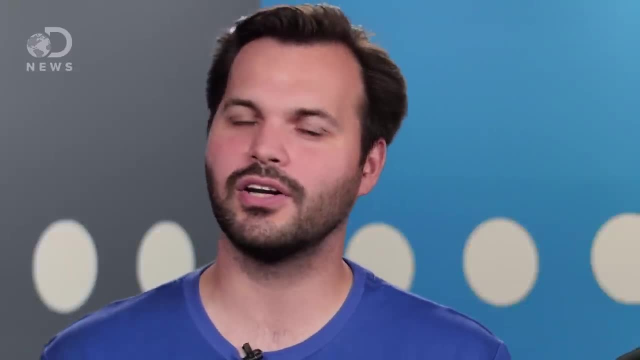 But according to the Standard Model there is no crossover And since the proton is the lightest baryon, it should be stable. After all, you can't just create something heavier. But scientists are an inquisitive bunch. maybe you've heard. 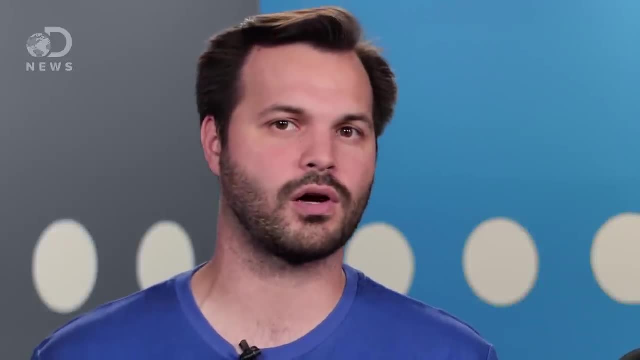 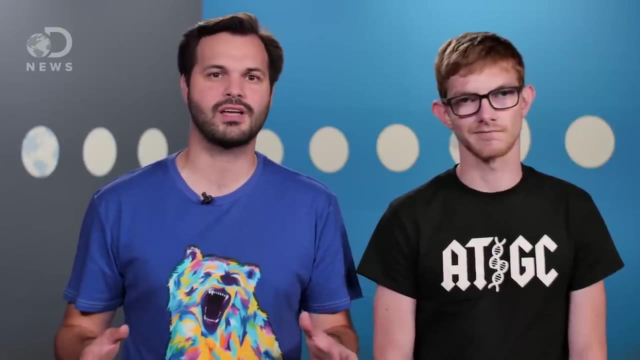 And in the 1970s they noticed that these sixteen different forms of quarks were not all the same. They all had different colors and up and down spins could fit together. We talked to particle physicist Keith Dines from the National Science Foundation and 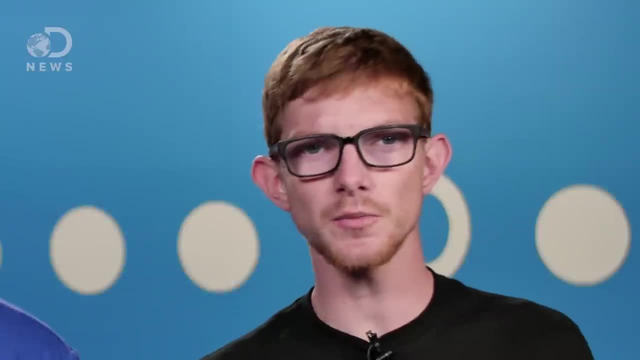 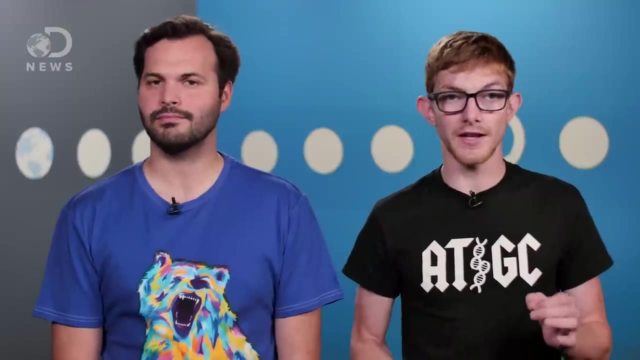 he explained that it's sort of like jigsaw pieces And when you put a jigsaw together you get a new picture And the picture spreads across all the pieces. That means that if there is a grand unified theory, then baryons and leptons are connected. 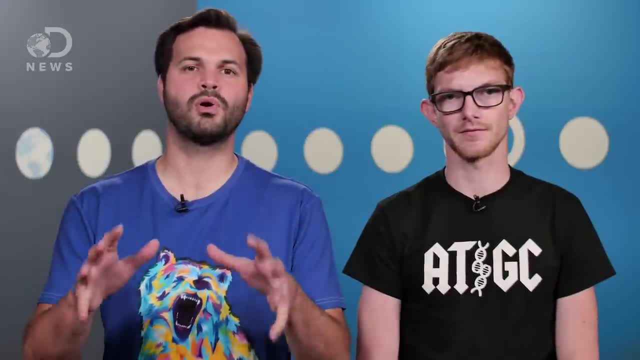 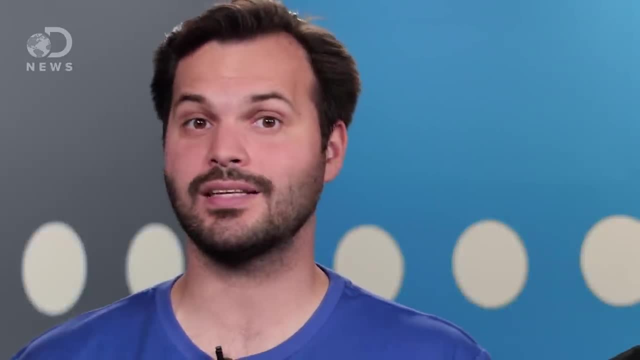 and one should be able to become another. That's where proton decay comes in To bring it all back. If we watch and we wait and we get really, really lucky, we might witness a proton decaying, And if it does, this means there is something beyond the Standard Model of Physics, aka. 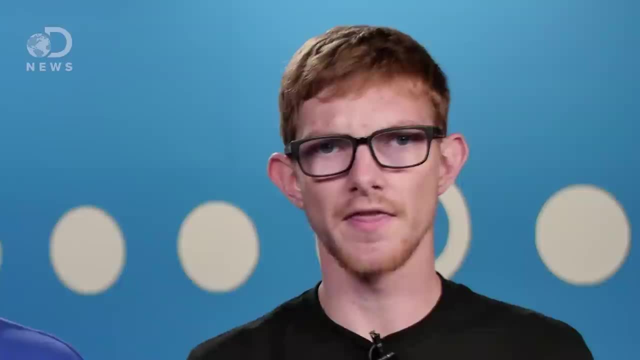 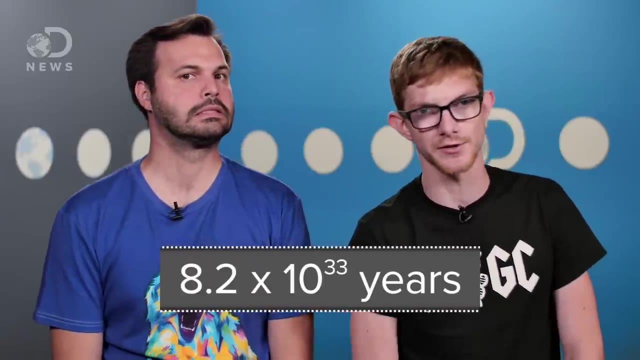 the explanation of particle physics that every single experiment ever supports. They might have to wait a while, though, as the half-life of a proton is estimated at 8.2 times 10 to the 33 years, That's 8 million billion, billion billion years. 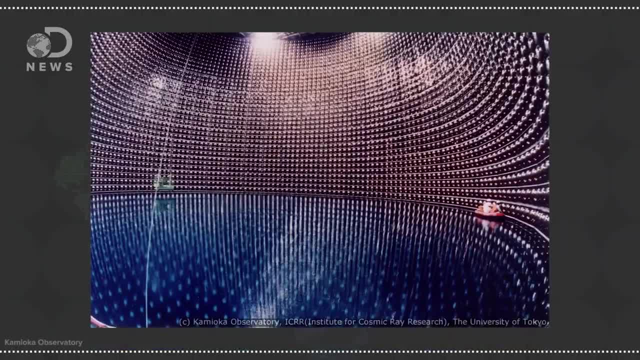 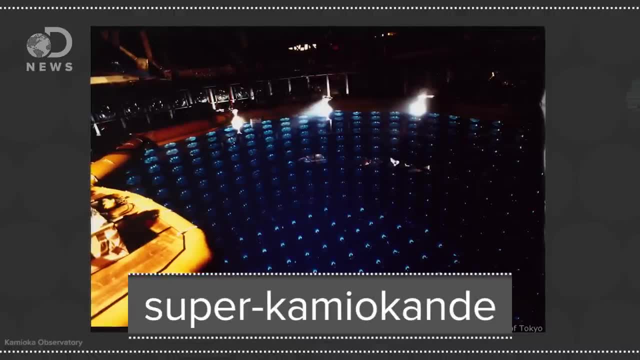 So right now, 1,000 meters under a mountain in Japan, there is a tank Of 50,000 people And tons of ultra-pure water. This water tank, known as Super-Kamiokande, is watching that H2O.